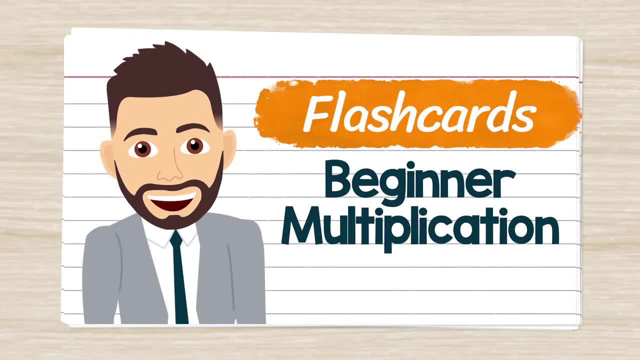 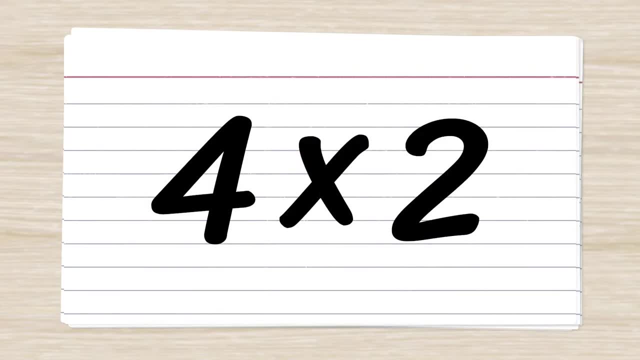 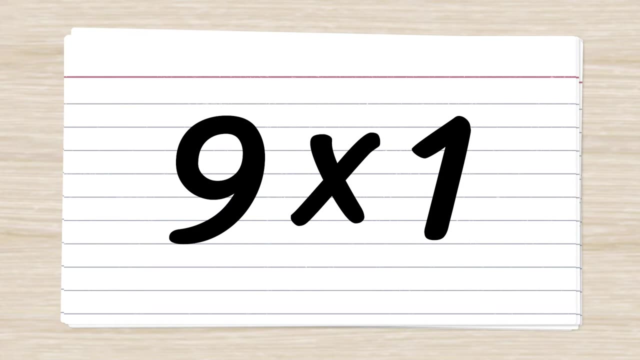 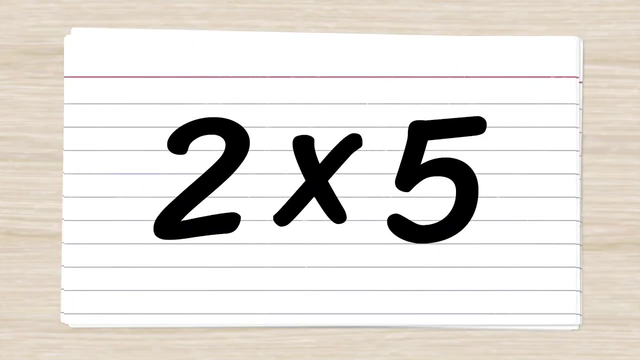 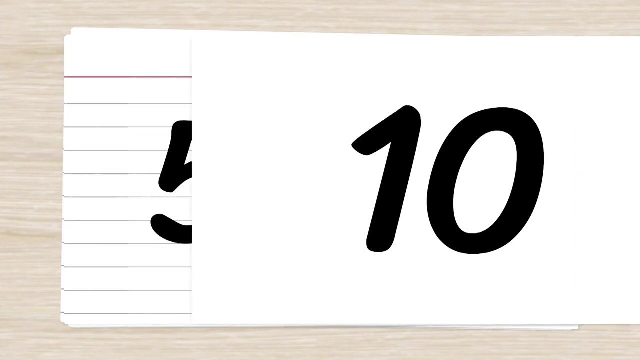 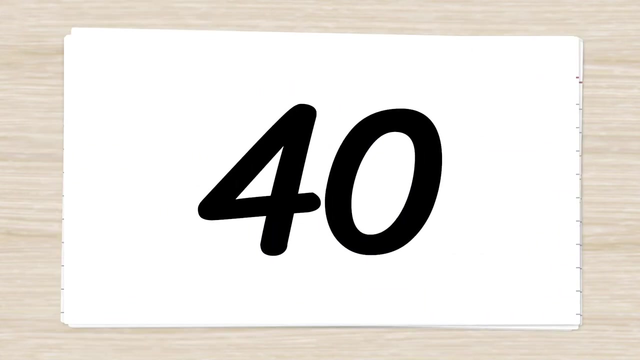 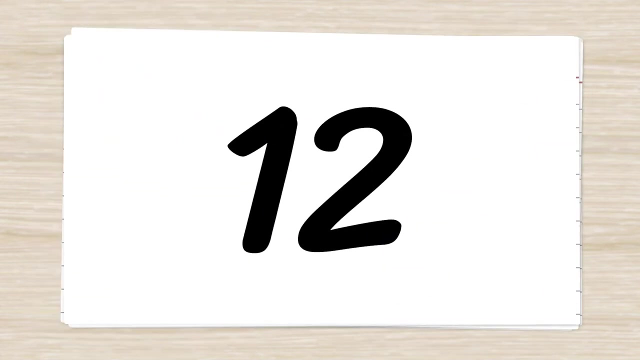 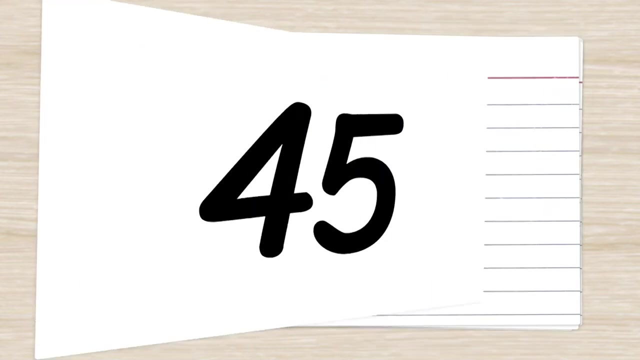 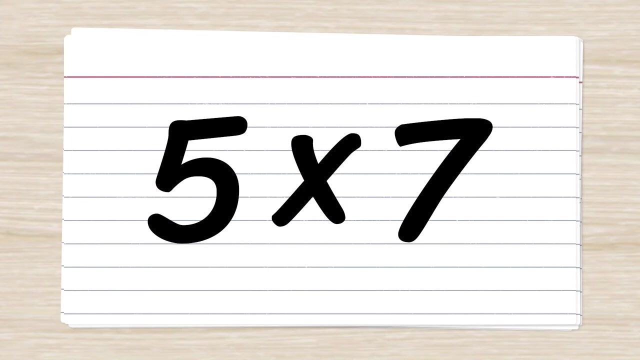 Welcome to Multiplication Flashcards with Mr J, So I hope you're ready. Let's get started. Two times five, Ten, Five times eight. Forty, Three times four. Twelve, Nine times five, Forty, Forty-five, Five times seven. Thirty-five Two times nine, Eighteen, Four times four. Sixteen, Eight times nine. 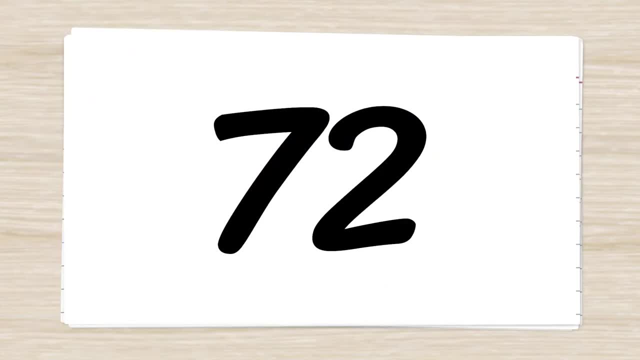 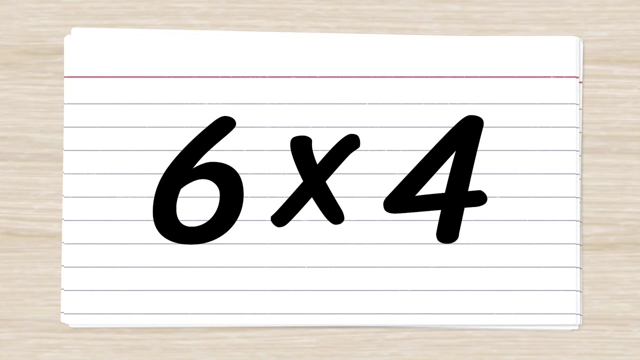 Seventy-two Nine times three. Twenty-seven, Seven times two. Fourteen Six times four. Twenty-four, Three times three. Sixteen, Nine, Four times four. Sixteen Five times five. Twenty-five Eight times two, Sixteen.